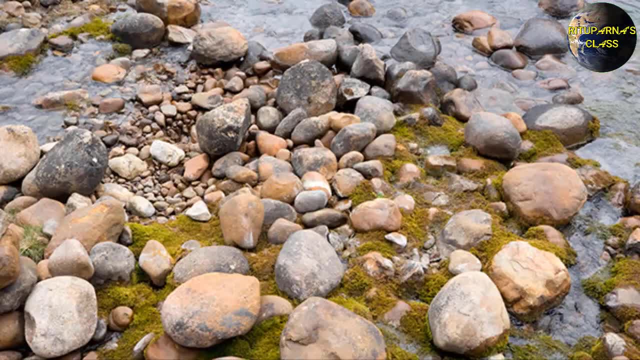 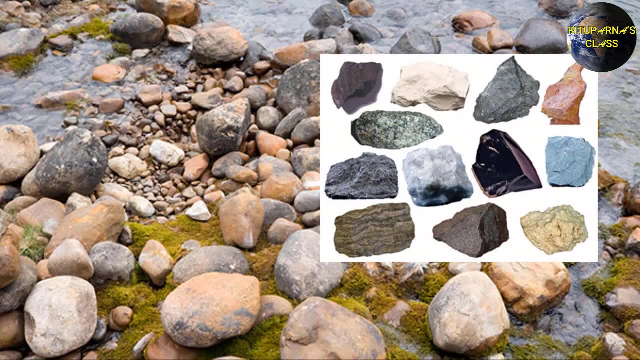 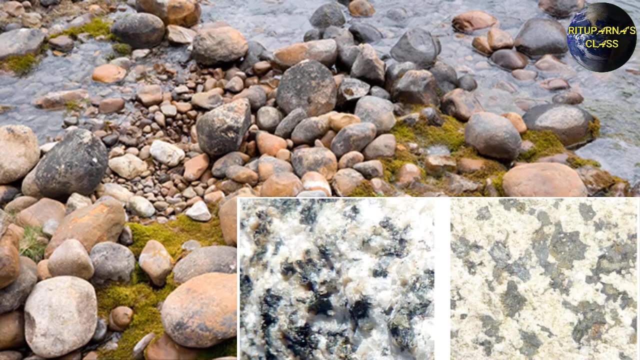 what is chemical weathering? If you look at any rock collection, you may see rocks of all different shapes, sizes and colors. Some of these differences might be the result of weathering, which is when rocks are broken down into smaller pieces or changed to the point where they become. 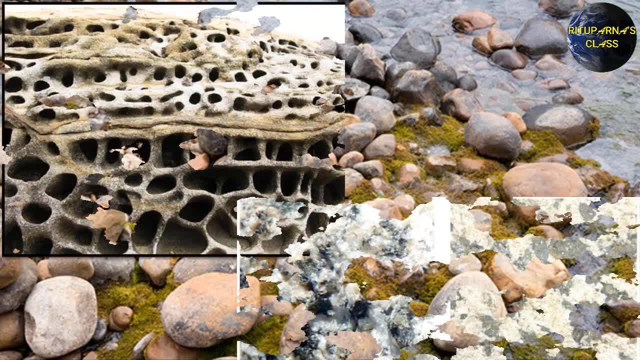 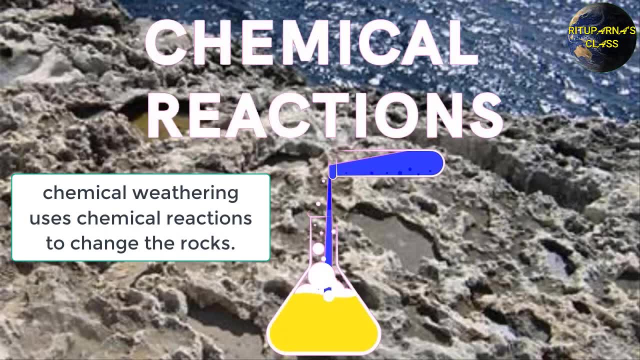 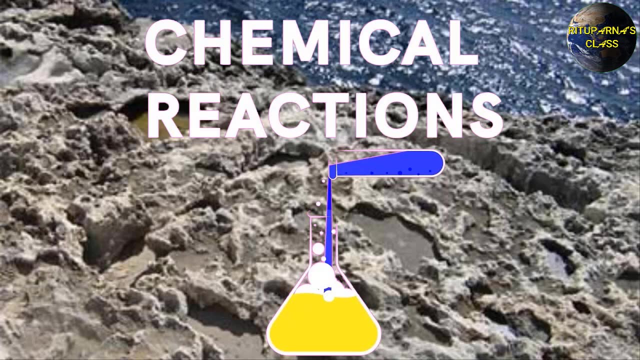 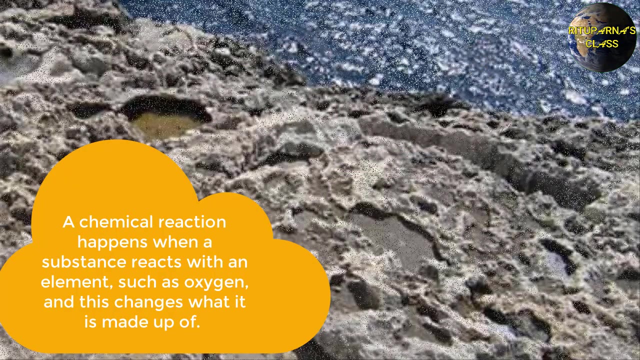 a different type of rock. This type of weathering is called chemical weathering. Chemical weathering uses chemical reactions to change the rocks. A chemical reaction happens when a substance reacts with an element such as oxygen and this changes what is made up of. The result is a substance made up of new elements. 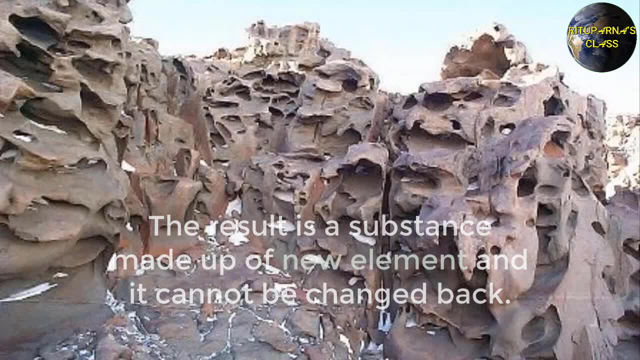 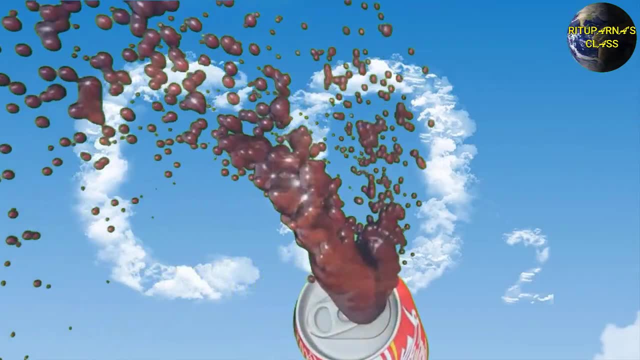 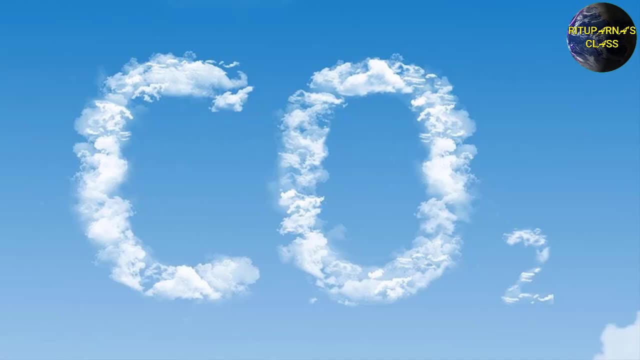 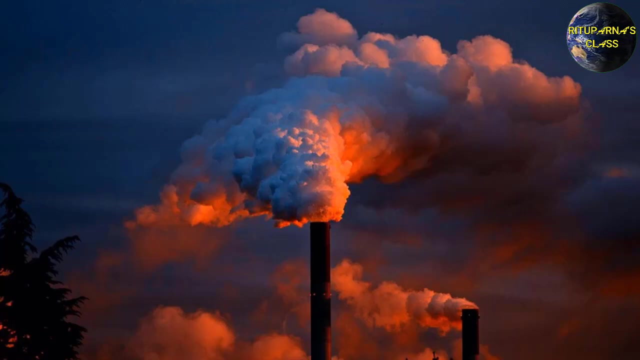 and it cannot be changed back. When you take a drink of soda, you hear a sound. when you open a bottle of soda, You are feeling and hearing carbon dioxide being released. Carbon dioxide and other chemicals are also released into our atmosphere because of the pollution from cars and factories. This results in something known as acid rain. 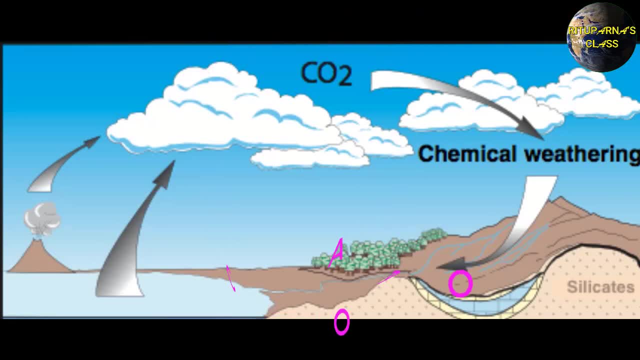 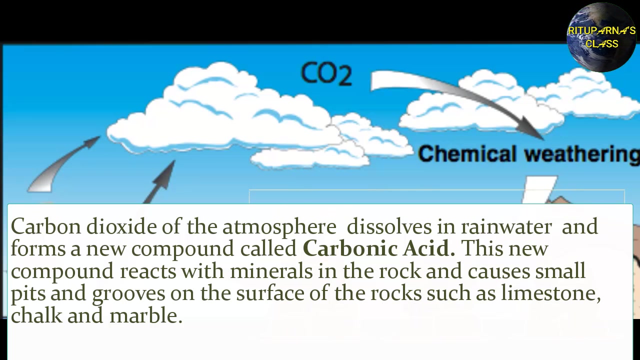 It doesn't usually hurt plants or animals, but it can affect rocks. Carbonation happens when this acid rain combines with rocks and changes the way they are formed. So we can say this occurs when carbon dioxide in the atmosphere dissolves in rain water and forms a new compound called. 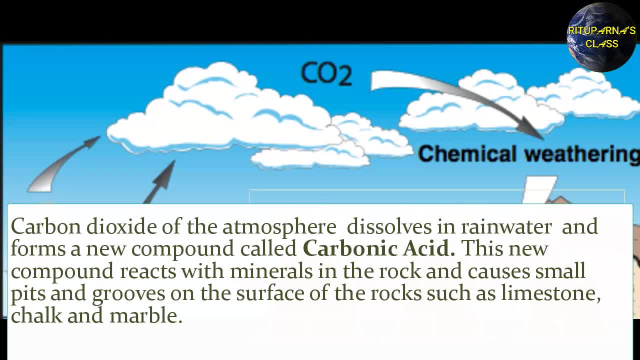 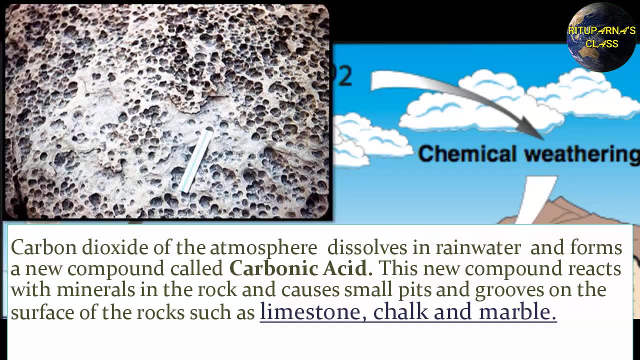 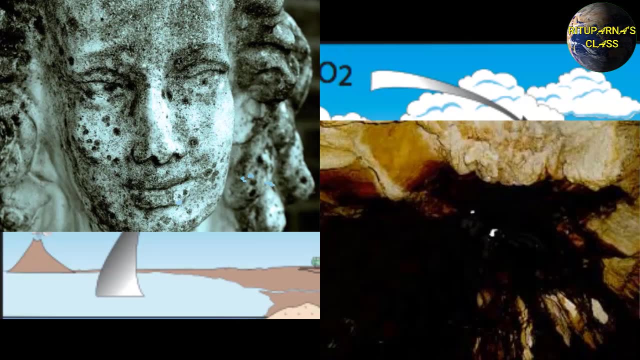 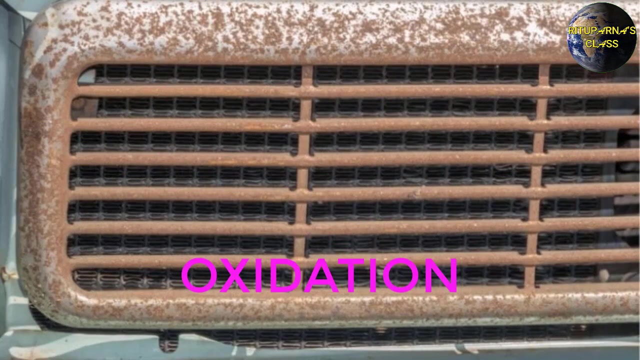 carbonic acid reacts with minerals in the rocks and causes small pits and groups on the surface of rocks such as limestone, chalk and marble. Here you can see few examples of carbonation. Have you ever left your bike or any metal toy outside for a few weeks? 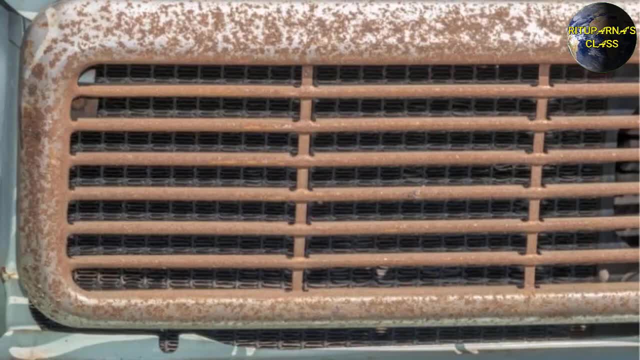 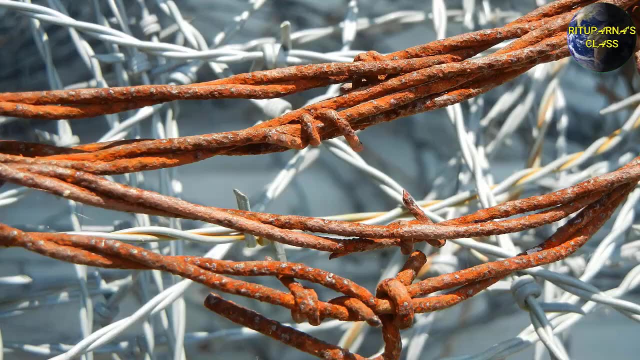 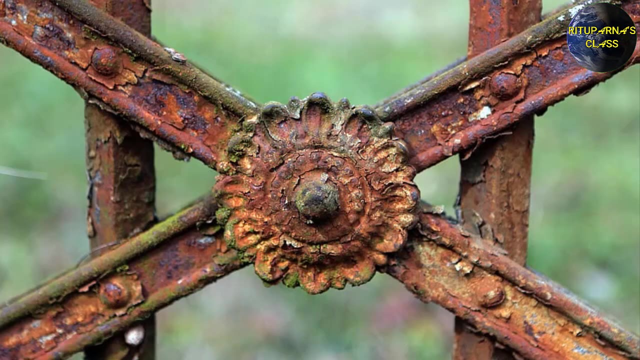 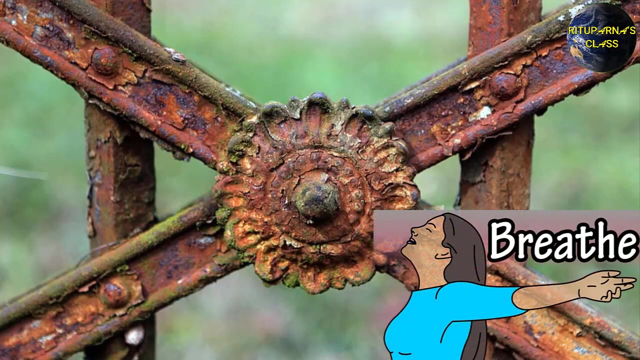 Did you notice that some of the metal parts turned red or rusted? If you leave it outside for a very long time, it may even start to break apart. This happens because that metal was exposed to an element we need to survive, So Oxygen is playing a major role here. 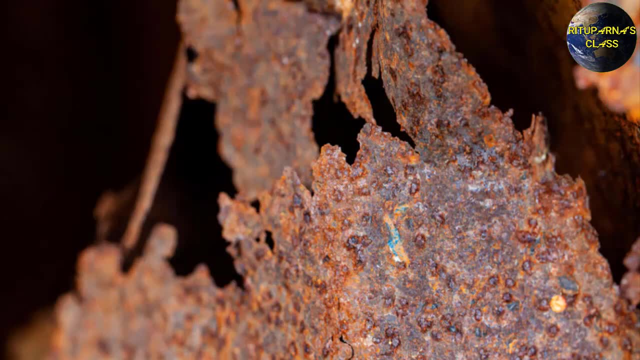 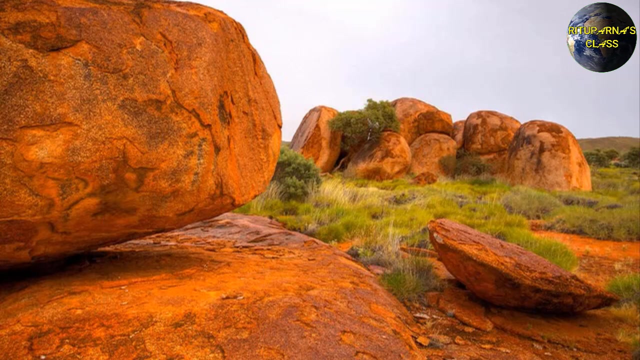 It is some of the most abundant, something so valuable to us but can be so destructive. Now, in this process, oxygen in the air reacts with certain minerals in some rocks, resulting in the formation of a new chemical compound which is far more easily eroded. 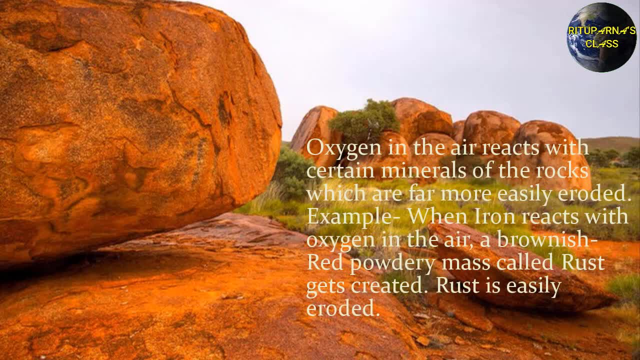 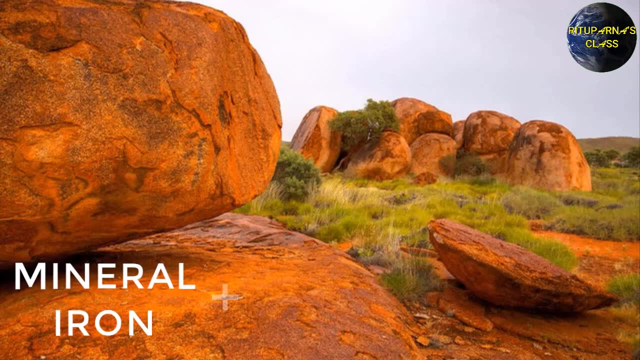 This weakens the rocks. For example, many rocks contain some amount of the mineral iron. When iron absorbs oxygen from the air, it rusts, changes its color and becomes a brown or red powdery mass called rust, which is easily eroded. 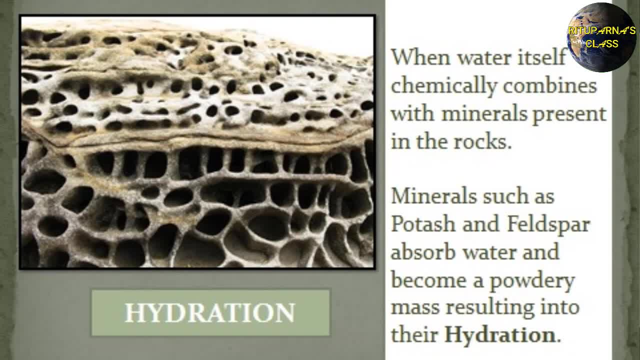 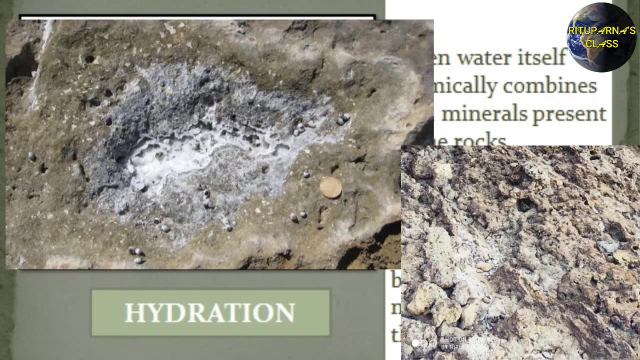 Next is Hydration. This occurs when water itself chemically dissolves. Hydration is chemically combined with. some minerals present in rocks, such as feldspar and potash, absorb water and become a powdery mass due to the process of hydration resulting. 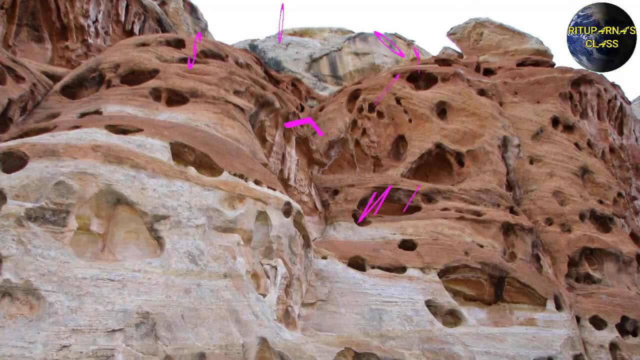 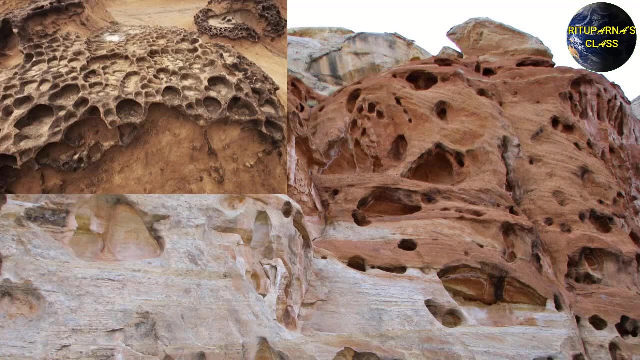 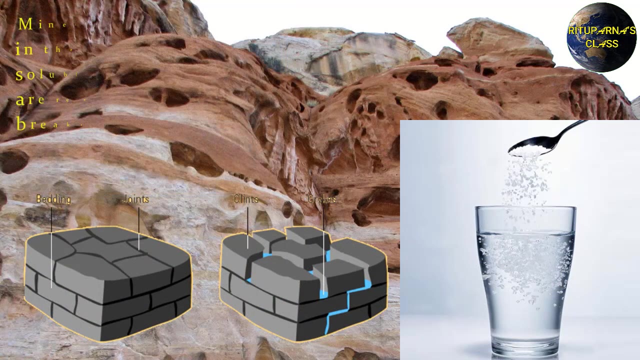 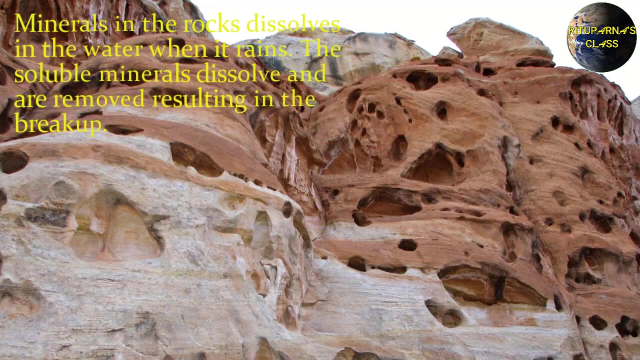 in their erosion. Next, this is the simplest form of chemical weathering, by which some minerals in the rocks dissolve in water. When drained water falls, Soil falls on these rocks or when river flows over them, the soluble minerals dissolve and are removed, resulting in the breakup of rocks. 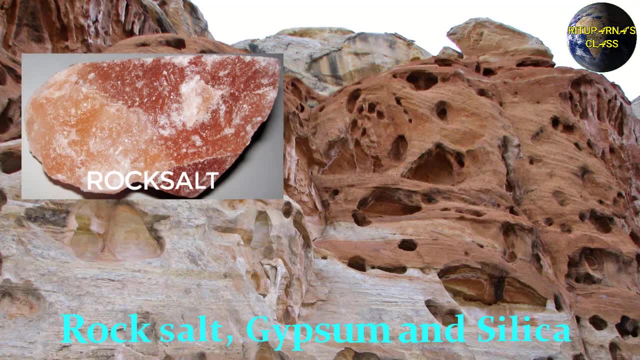 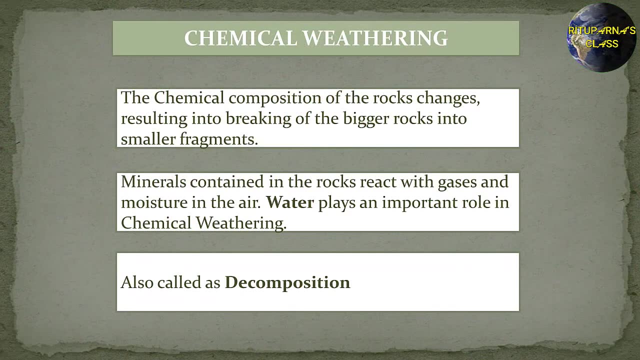 Rock. salt, gypsum and silica are few examples of minerals that are highly soluble. So at the end we can say: chemical composition of the rocks: changes resulting in the erosion of the rocks. So at the end we can say: chemical composition of the rocks: changes resulting in the erosion. 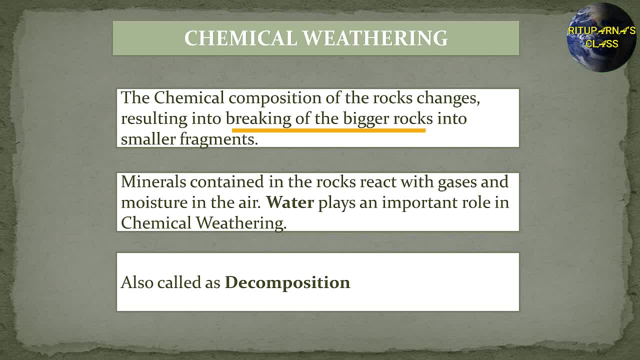 of the rocks. So at the end we can say chemical composition of the rocks changes into breaking of bigger rocks into smaller fragments. Minerals contained in the rocks react with gases and moisture in the air, where water plays an important role, and chemical weathering, also called decomposition.